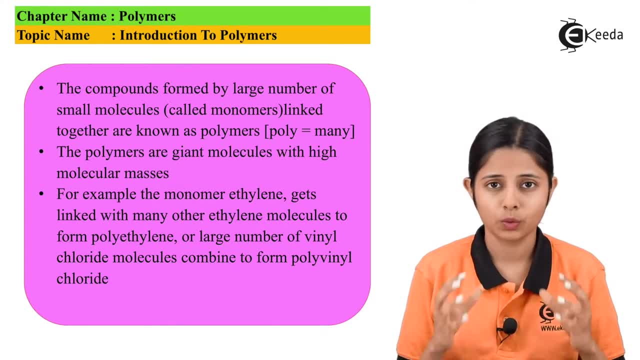 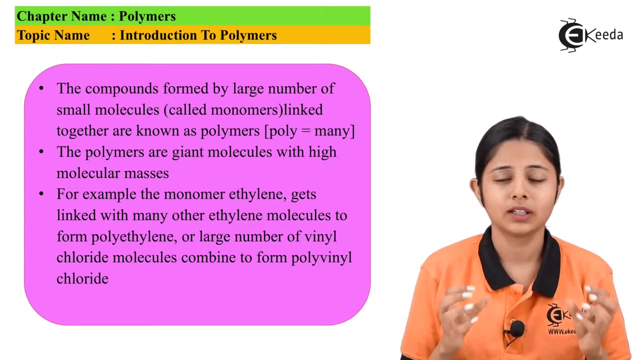 know that these are polymers. they do not look huge. they do not look big but they have certain properties in them and those properties make these polymers extremely desirable for high utility. polymers are nothing but giant molecules and these giant molecules, giant compounds and substances containing molecules coming together. let us take an example of polythene. 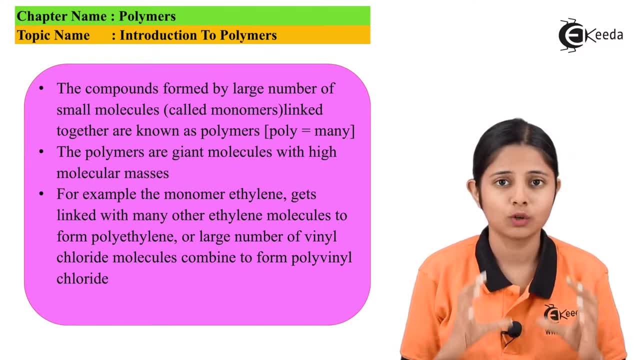 polythene bags are common in use. polythene bags are those plastic bags which we use for carrying vegetables from the vegetable vendor to home. these polythene bags are made up of ethene. ethene is nothing but an alkene. what is an alkene? a carbon with another carbon, and both these. 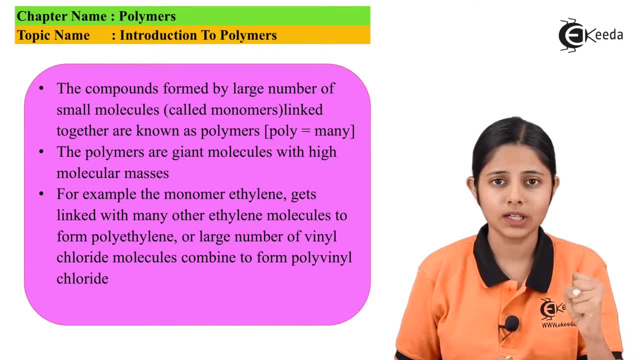 carbons are bonded with a double bond. so this is my one carbon, this is my another carbon, and both these carbons have two bonds in the middle. these two bonds state that it is an alkene and this two carbon state that it is an ethene. so when i take this ethene, i break the second. 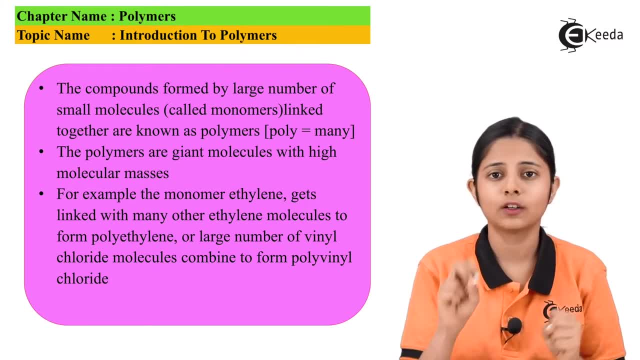 bond out of it, then these two carbons will get two more valencies. that means this carbon can make one more bond. this carbon can also make one more bond and because of that they go and join together with two other carbons. that means many ethens come together. 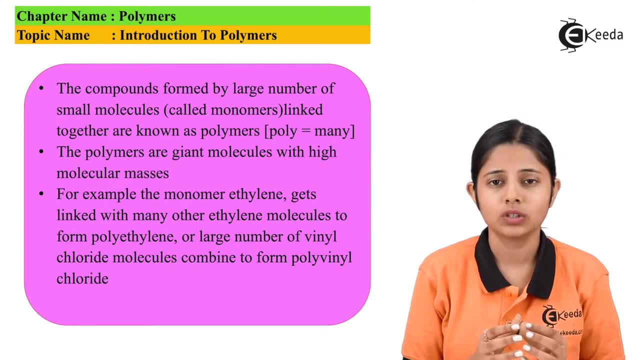 they break their second bond. and after breaking the second bond, this ethens club in together to form a long chain of carbon. this long chain of carbon is known as polyethene, which now we call as polythene bags. this is nothing but a polymer or a plastic. so now in. 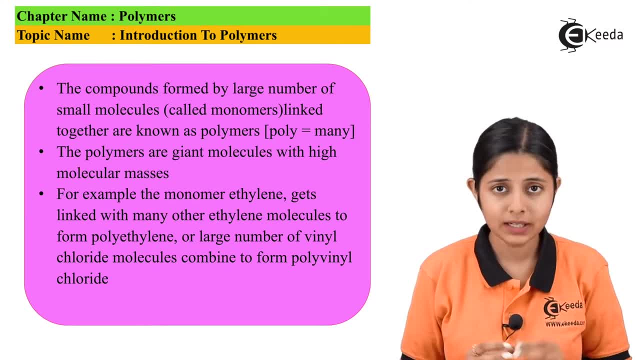 my polymers. what is the monomer? monomer is the single repeating unit which will keep on repeating itself and keep on clubbing together with other such monomers to finally form a polymer. now, for example, in polyethene box, that is, polythene bags, the ethene, that is one carbon with another carbon and both the carbons. 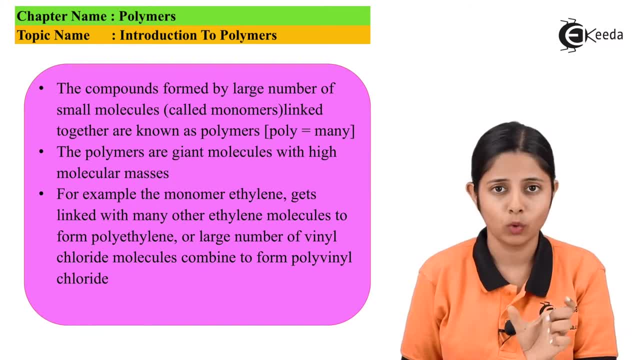 club together or join together with a double bond, becomes my monomer. Now this monomer will club together with another such monomers. that means all the same monomers will come together and finally all of them will form a polymer. Monomers combine together to form polymers In polyethene. 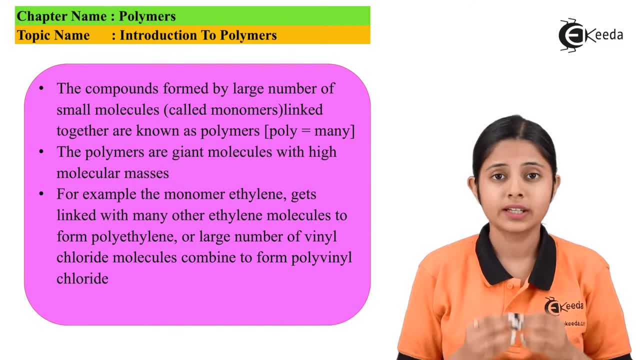 the ethene molecule is the monomer. Now there is a comparison or a classification between the polymers itself. There are certain polymers which have high degree of polymerization. There are other such polymers which have low degree of polymerization. Now, what exactly is? 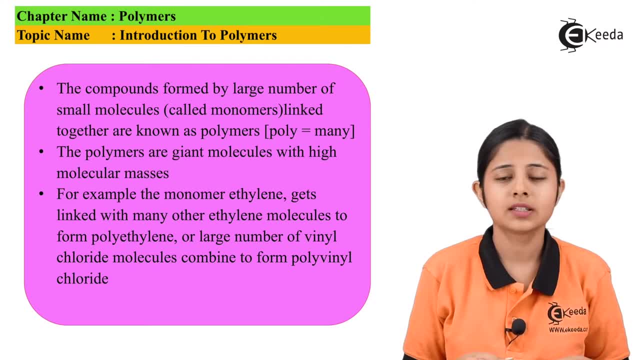 degree of polymerization. The degree of polymerization is the property by attributes of which the carbon or any other monomer can form chains together. That means, if many monomers come together to form a monomer, then the monomer will be a monomer. Now this monomer is a monomer. 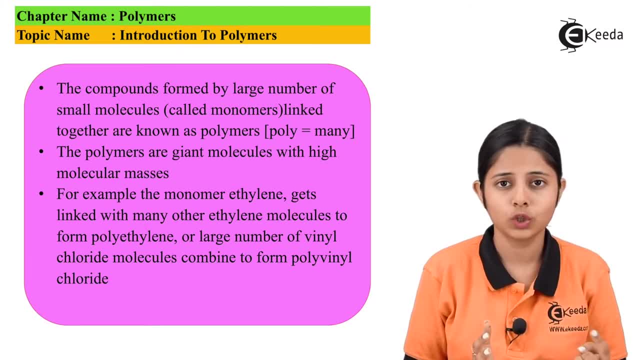 It can also form a molecule over here and these chains are joined together. that is high degree of polymerization. There are certain other molecules wherein many monomers cannot club in together. There are low level of monomers with low molecular mass. that is low degree of. 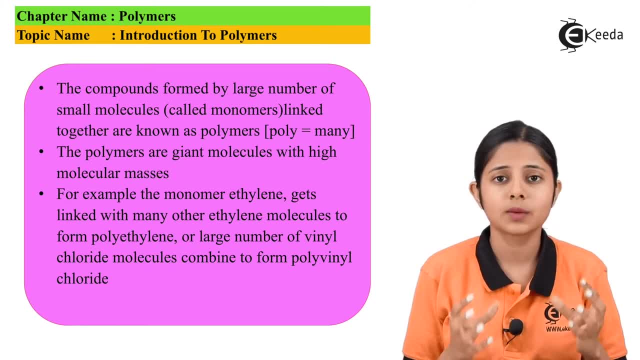 polymerization- High degree of polymerization. the substances which go through the high degree of polymerization, which have the ability to go through the high degree of polymerization, are known as my normal polymers, And the substances which do not go high degree of polymerization, that means which will go through low degree of polymerization. 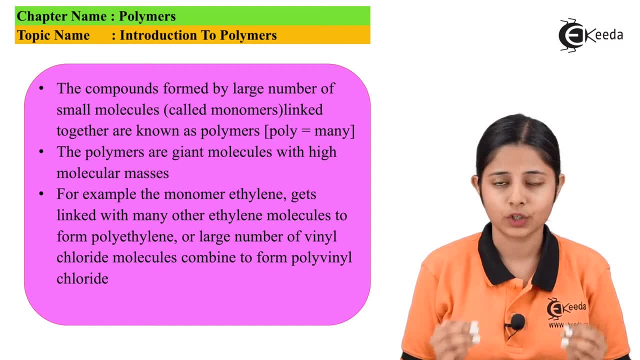 are known as oligomers. This is the basic classification between my polymers based on the properties of polymerization. that is, high polymerization are polymers and low polymerization are oligomers. So over here in today's session we studied about polymers. What exactly are polymers? 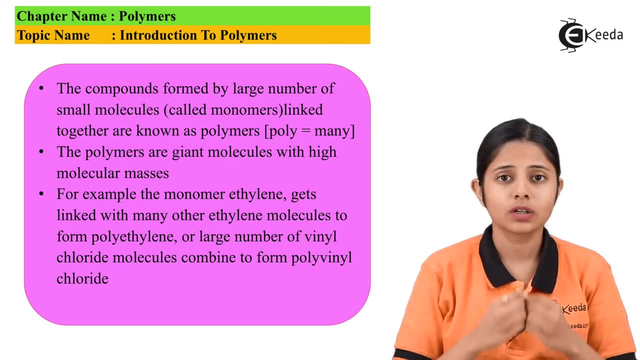 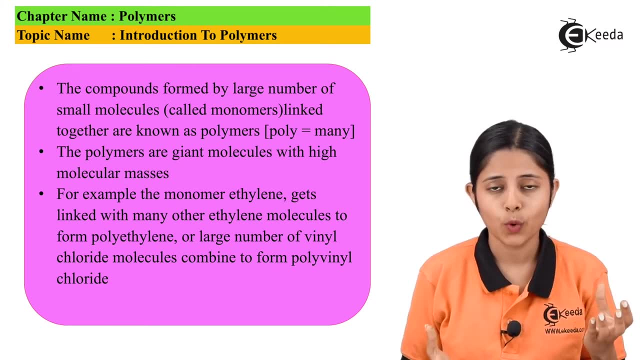 What are they made up of? They are made up of monomers. We also classified them on the basis of high polymerization and low polymerization. So we have a lot of polymers here. We have a lot of polymerization, high polymerization polymers and low polymerization oligomers. We took an example of 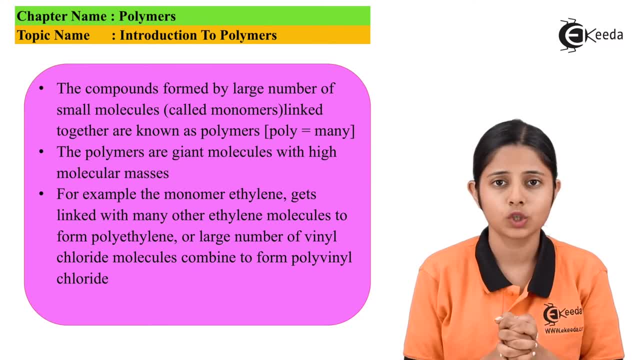 polythene. We took the monomer. We clubbed many monomers together in polythene. The monomer of polythene was ethene And over here many ethenes clubbed together and formed long chains to finally form the polythene that is the polymer. Thank you so much for watching this video. Stay tuned to. 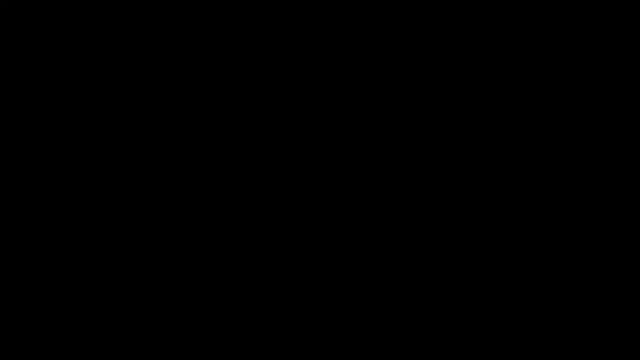 IKIDA and subscribe to IKIDA IKIDAcom.